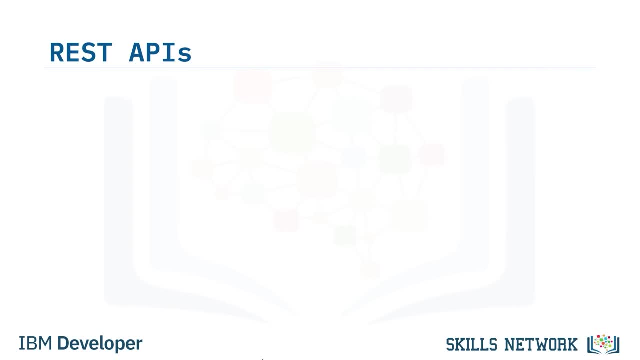 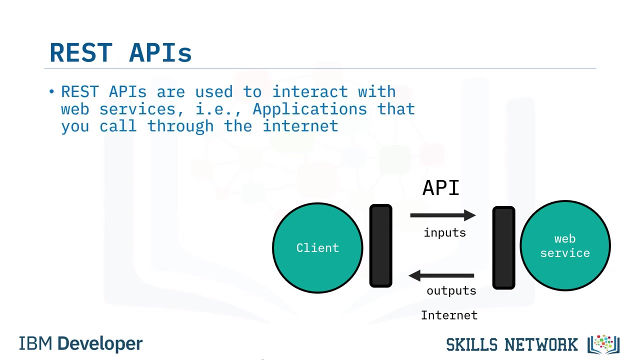 letting you take advantage of resources like storage access, more data, artificial intelligence, algorithms and much more. The RE stands for Representational, the S for State and T for Transfer In REST APIs. your program is called the Client. The API communicates with the API. 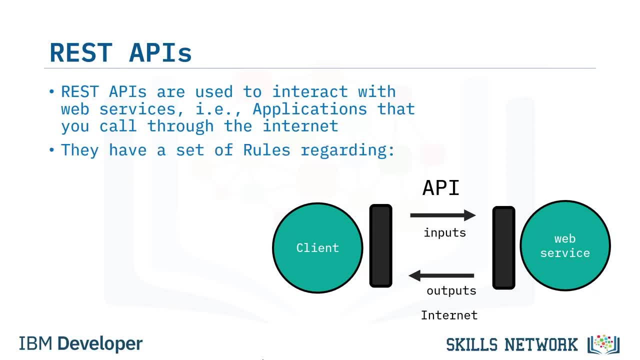 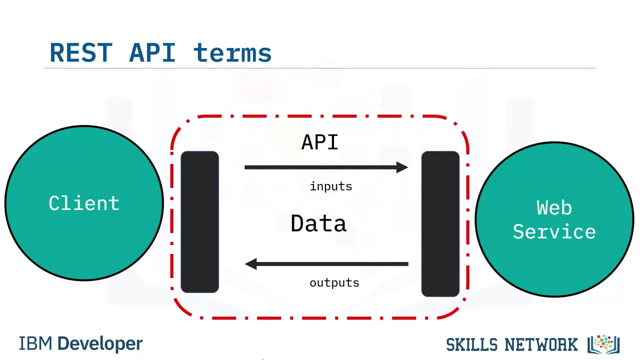 and communicates with a web service you call through the internet. There is a set of rules regarding communication: input or request, and output or response. Here are some common terms. You or your code can be thought of as a Client. The web service is referred to as a Resource. 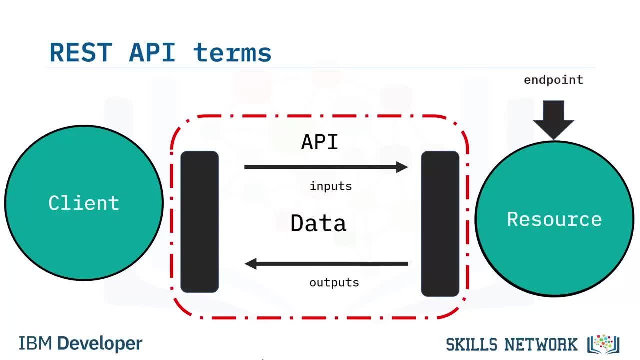 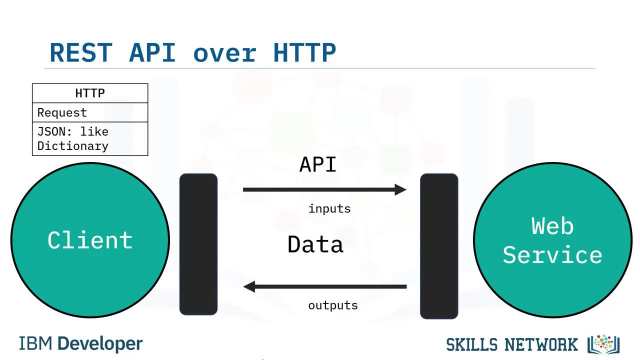 The Client finds the service via an endpoint. We will review this more in the next section. The Client sends requests to the Resource and the response to the Client. HTTP methods are a way of transmitting data over the internet. We tell the REST APIs what to do by sending a request. 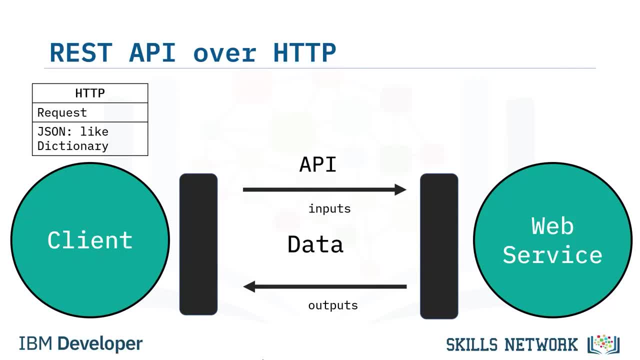 The request is usually communicated via an HTTP message. The HTTP message usually contains a JSON file. This contains instructions for what operation we would like the service to perform. This operation is transmitted to the web service via the internet and the service performs the operation. 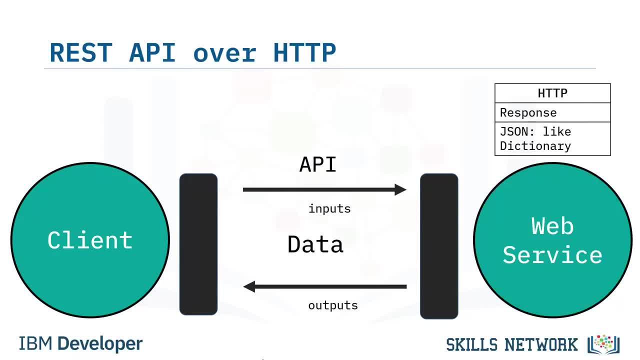 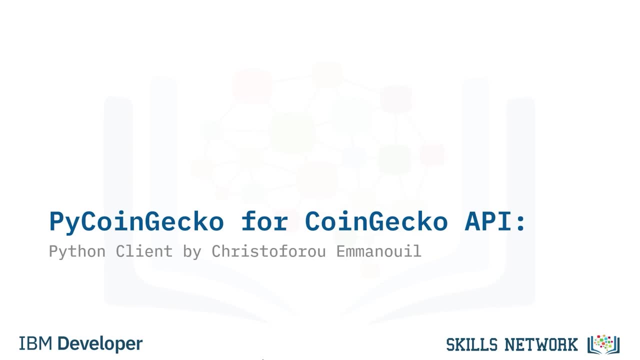 In a similar manner, the web service returns a response via an HTTP message, where the information is usually returned via a JSON file, and this information is transmitted back to the Client. Cryptocurrency data is excellent to use in an API because it is constantly updated and is vital to cryptocurrency trading. 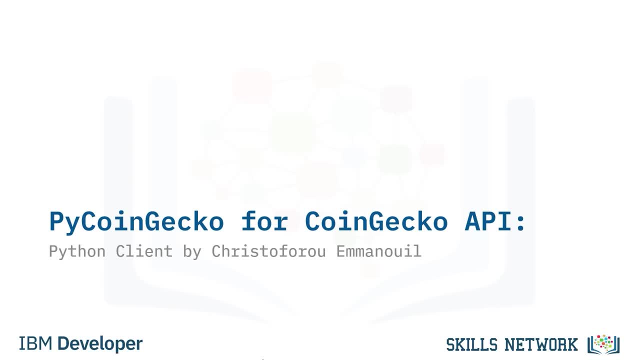 We will use the PiCoinGecko Python Client or Wrapper for the CoinGecko API, updated every minute by CoinGecko. We use the Wrapper or Client because it is easy to use, so you can focus on the task of collecting data. 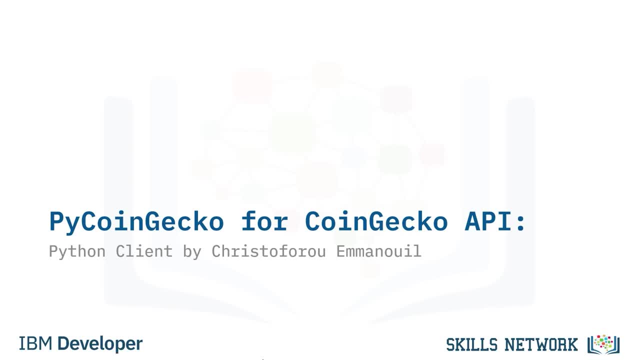 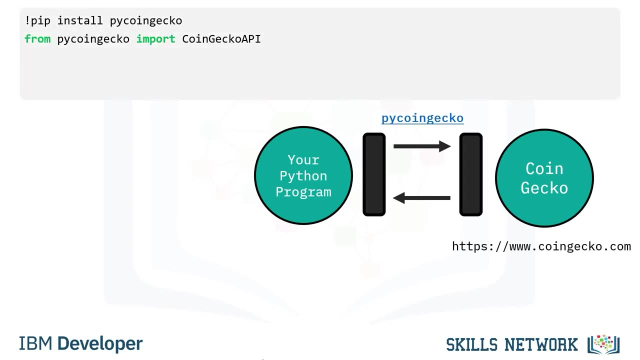 We will also introduce Panda's time series functions for dealing with time series data. Using PiCoinGecko to collect data is simple. All we need is to install and import the library, then create a Client object and finally use a function to request our data. 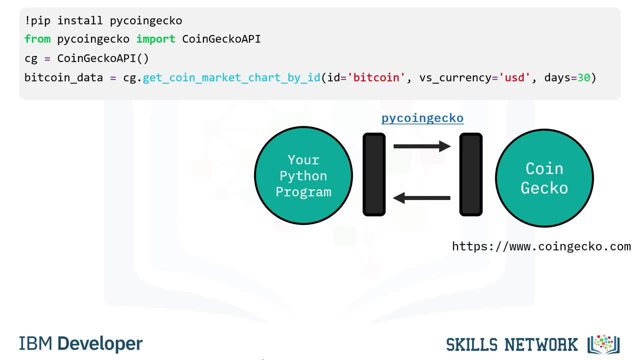 In this function, we are getting data on Bitcoin in US dollars for the past 30 days. In this case, our response is a JSON file expressed as a Python dictionary, of nested lists, including price, market cap and total volumes, which contain the Unix timestamp and the price at the time.